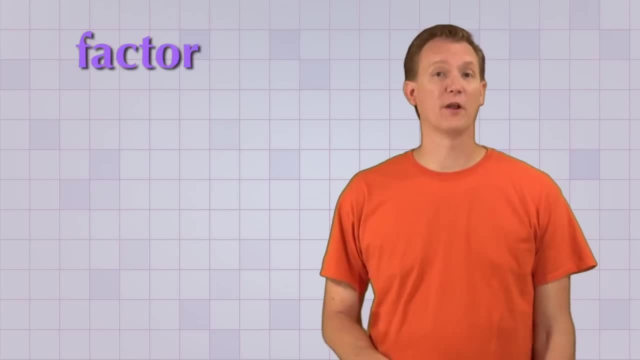 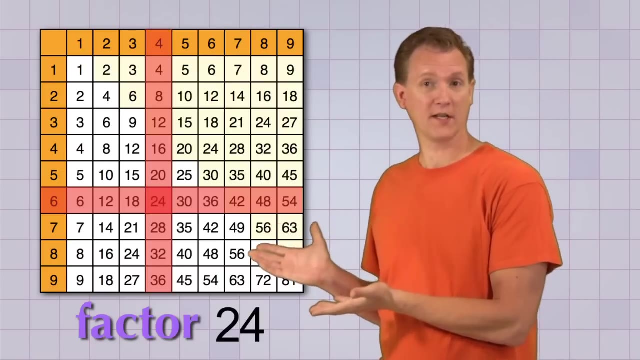 how to do it. So let's see another example. Let's factor the number 24.. For this one, I think I'll use my multiplication table. Let's see here: Alright well, 4 times 6 is 24.. So that means: 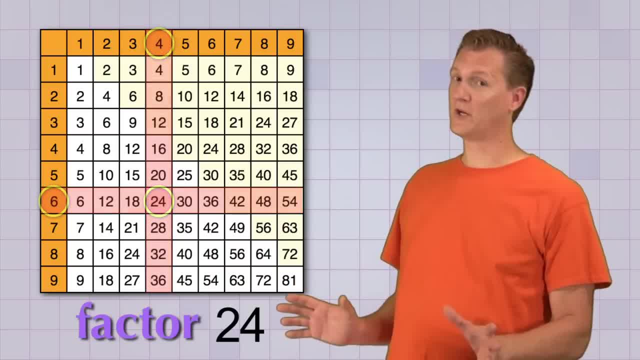 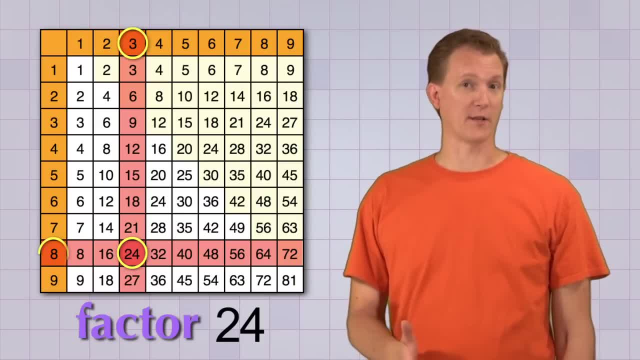 that 4 and 6 are factors of 24.. Now hold on. I'm sure some of you have seen that 3 times 8 is also 24. And that's true. We could have decided to factor 24 into 3 times 8 instead. 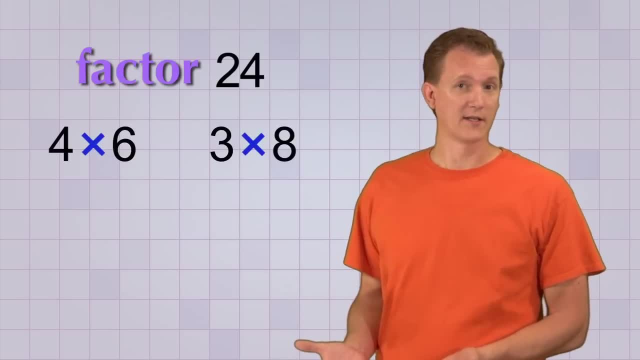 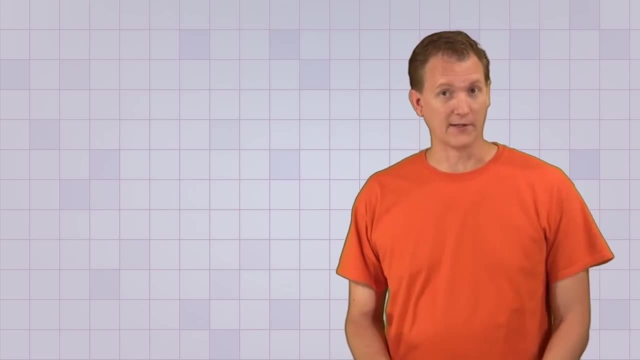 So which of the factors is right? Is it 4 and 6, or 3 and 8?? Actually, they're both right. There can be more than one way to factor a number. That's one of the things that might make factoring a little confusing. 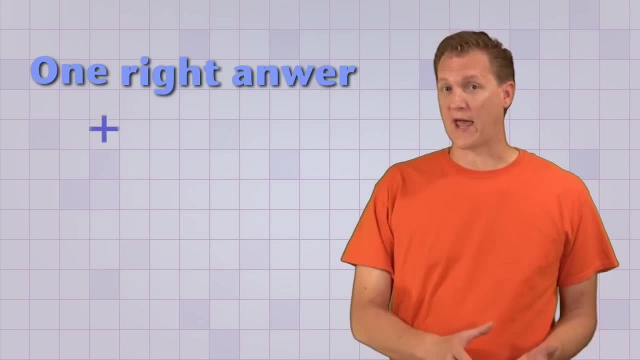 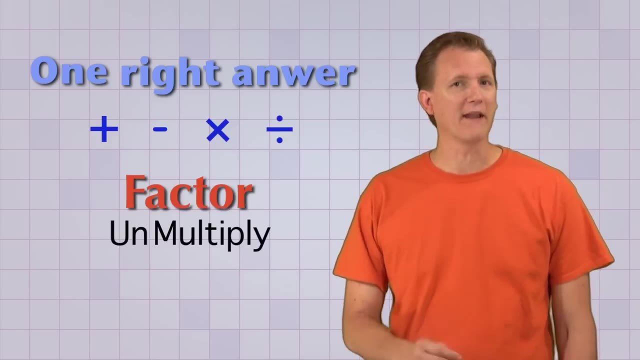 at first You're used to having just one right answer, Because when you add, subtract, multiply or divide, there IS just one right answer. But when you factor or unmultiply a number, you might find that there's more than one correct way you can do it. 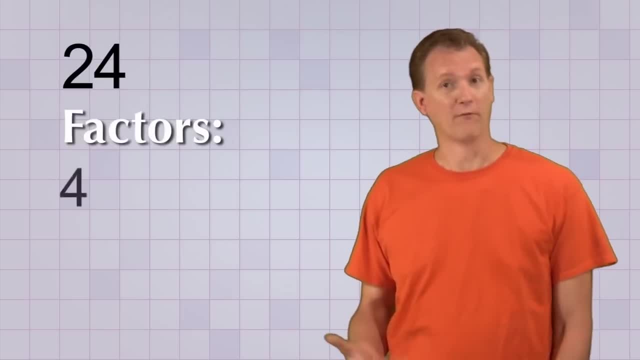 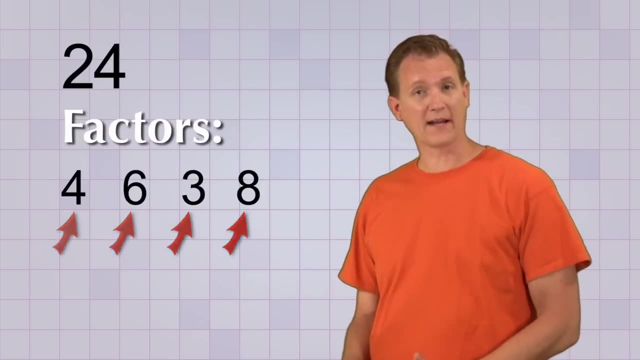 So we can see that the number 24 has quite a few factors: 4 is a factor, 6 is a factor, 3 is a factor and 8 is a factor. The fact that each of these numbers is a factor of 24 means that each 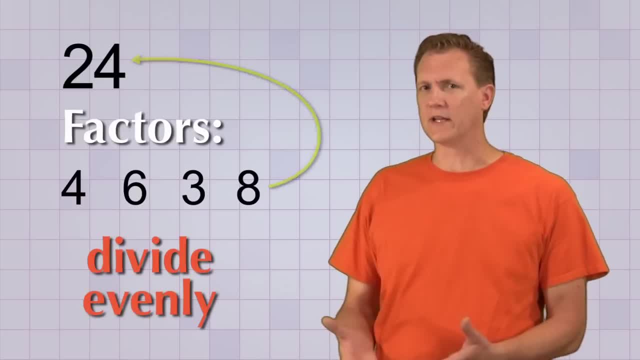 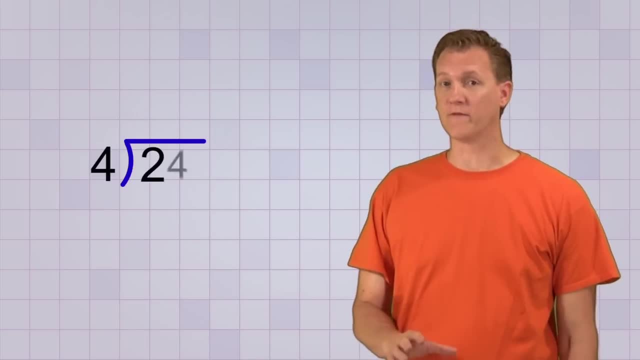 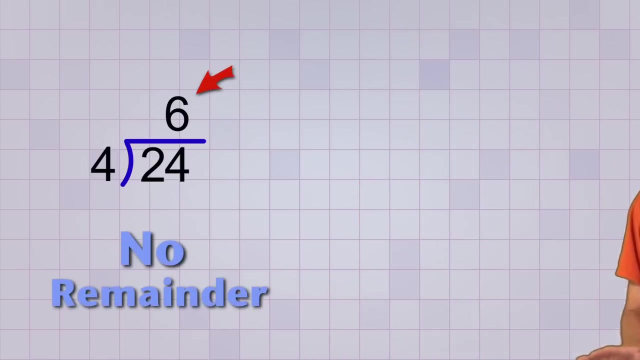 of them can divide evenly into 24.. And when I say divide evenly, I mean that it will divide in WITHOUT a remainder. For example, if we take our first factor, 4, and divide it into 24 using a calculator, our answer will be 6.. 4 divides into 24 6 times, with no remainder. But what if we try? 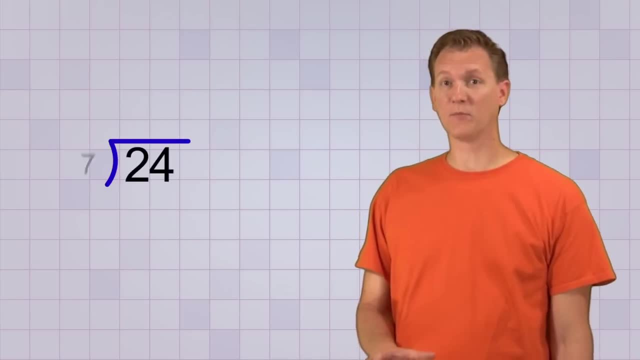 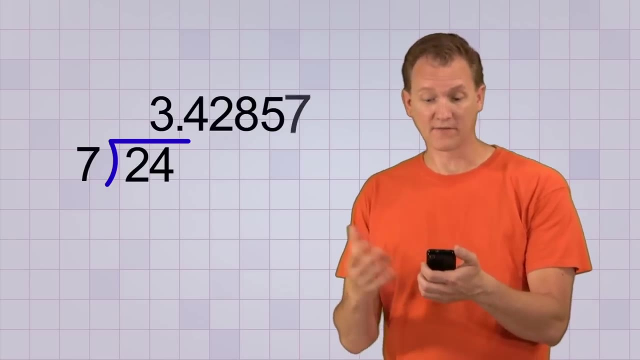 to divide 24 by a number that ISN'T one of our factors, like the number 7?? If we try to divide 24 by 7 on a calculator, we get 3.42857. blah, blah, blah- a long decimal number. 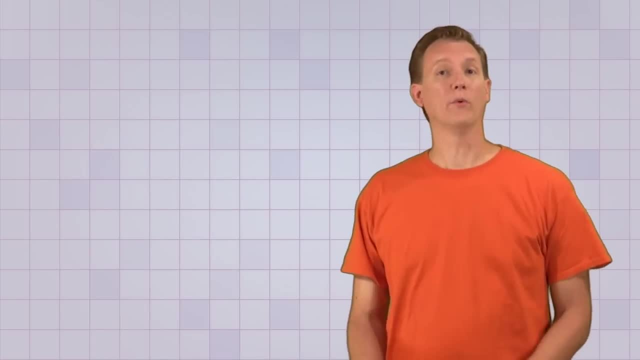 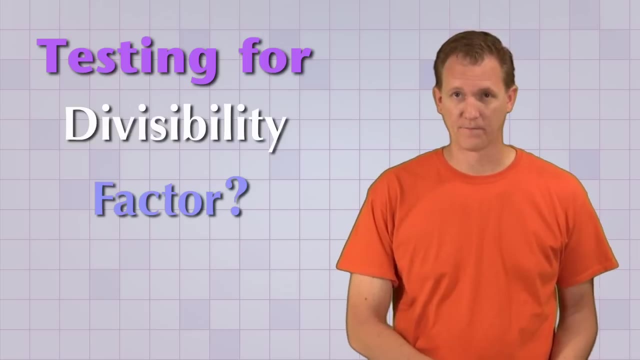 That didn't divide in evenly, because there's a big remainder. What we just did is called testing for divisibility. Testing for divisibility is a way to find out if a number is a factor of another number. With the test we just did, we confirmed that. 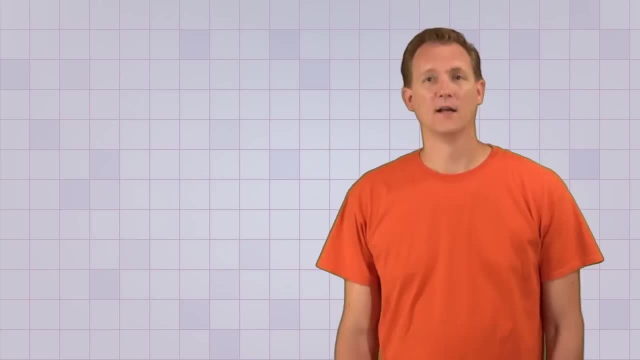 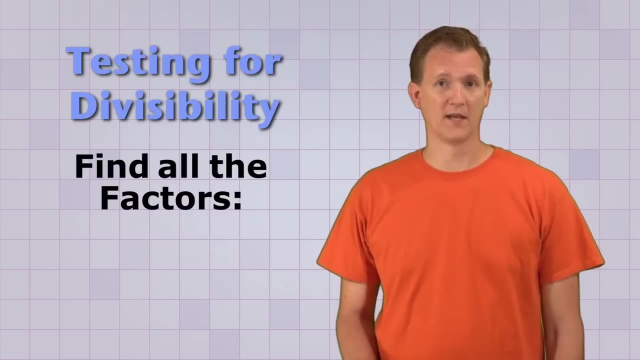 4 IS a factor of 24, but 7 is NOT. Sometimes you may be asked to find ALL the factors of a number. If that happens, you can use testing for divisibility To see how it works. let's try to find ALL the factors of 24.. 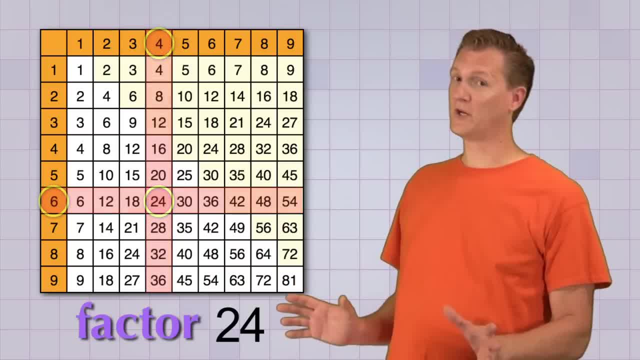 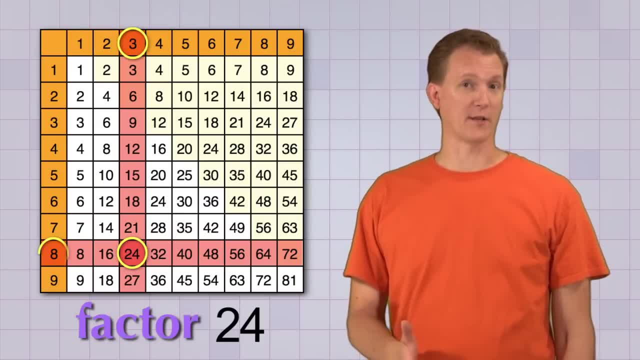 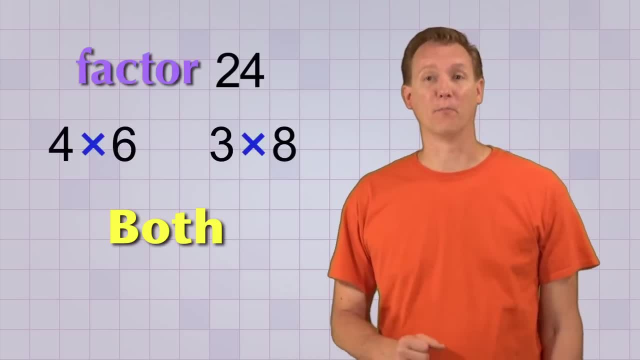 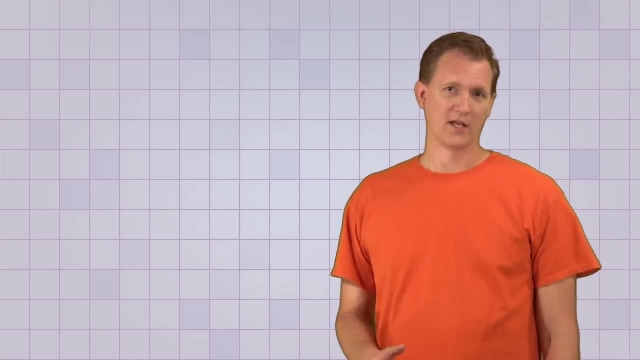 4 and 6? Or is it 3 and 8?? Actually, they're both right. There can be more than one way to factor a number. That's one of the things that might make factoring a little confusing at first, You're. 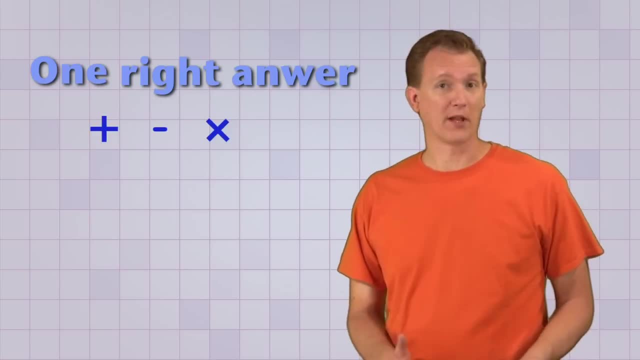 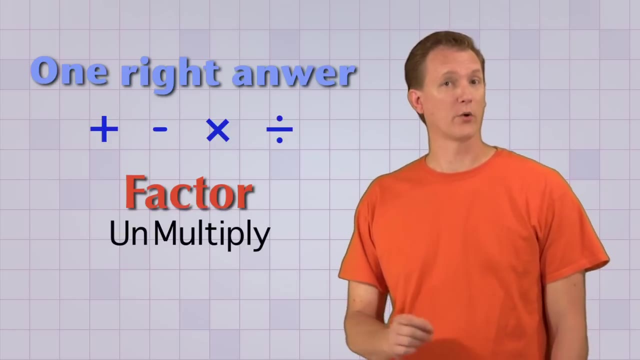 used to having just one right answer, Because when you add, subtract, multiply or divide, there is just one right answer. But when you factor or unmultiply a number, you might find that there's more than one correct way you can do it. 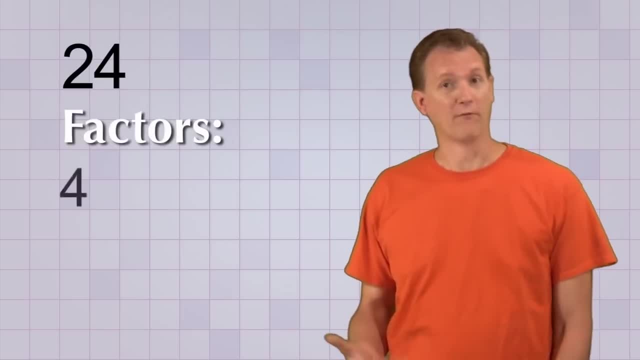 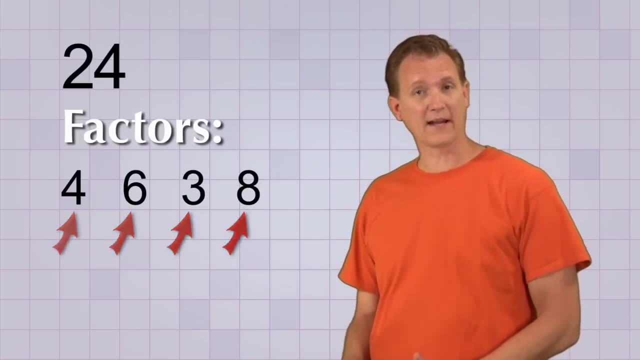 So we can see that the number 24 has quite a few factors: 4 is a factor, 6 is a factor, 3 is a factor And 8 is a factor. The fact that each of these numbers is a factor of 24 means that each of them can divide evenly. 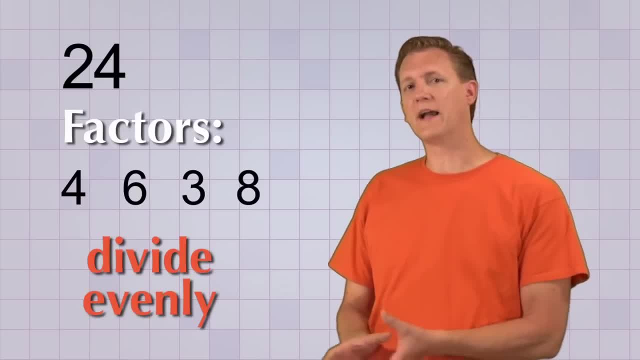 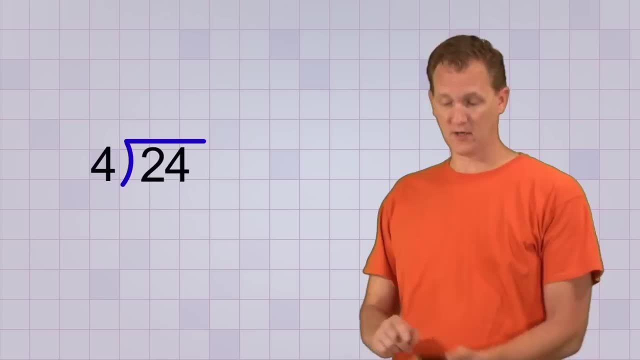 into 24.. And when I say divide evenly, I mean that it will divide in without a remainder. For example, if we take our first factor, 4, and divide it into 24, using a calculator, our answer will be 6.. 4 divides into 24, 6 times, with no remainder. 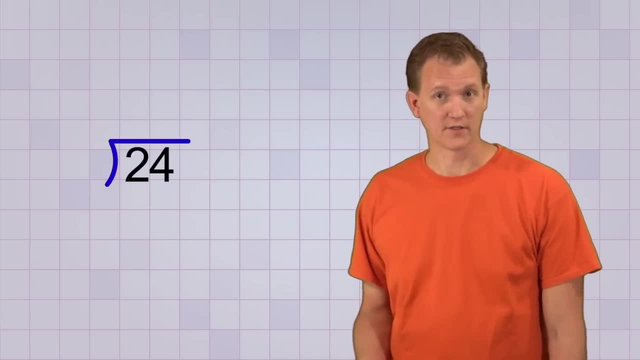 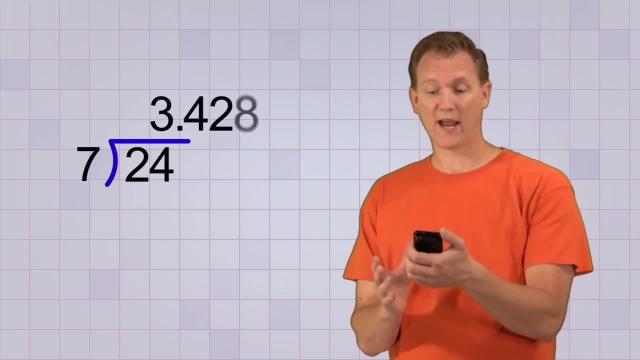 But what if we try to divide 24 by a number that ISN'T one of our factors, Like the number 7.. No, If we try 24 divided by 7 on a calculator, we get 3.42857. blah, blah, blah- a long decimal number. 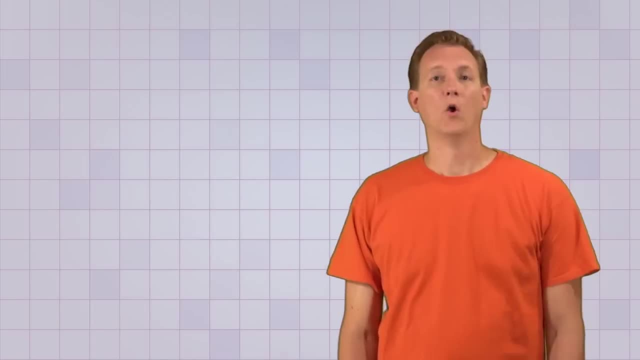 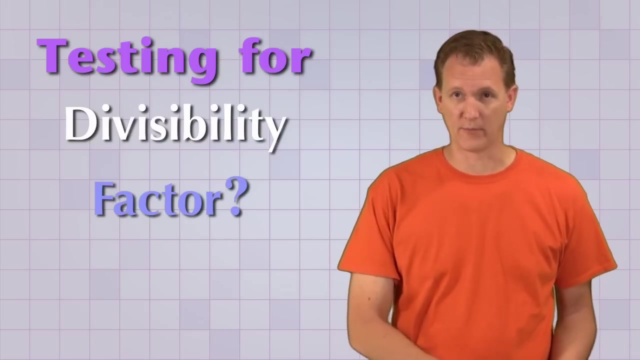 That didn't divide in evenly, because there's a big remainder. What we just did is called testing for divisibility. Testing for divisibility is a way to find out if a number is a factor of another number. With the test we just did, we confirmed that 4 is a factor of 24, but 7 is not. 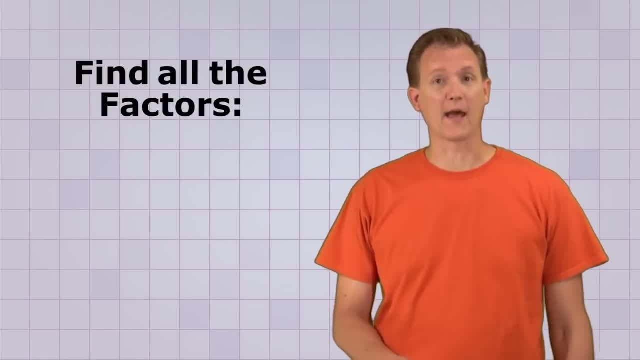 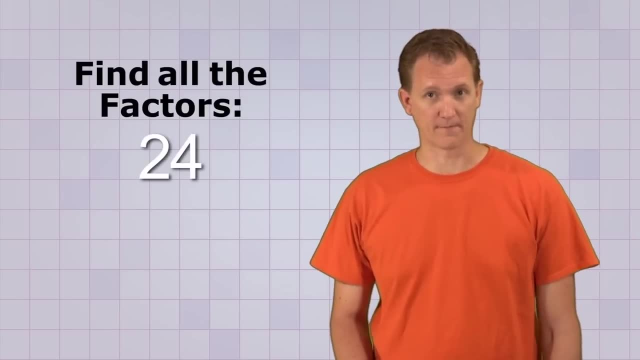 Sometimes you may be asked to find all the factors of a number. If that happens, you can use testing for divisibility to solve the problem. To see how it works, let's try to find ALL the factors of 24.. We already know 4 of them, but there are a lot more numbers we can test. 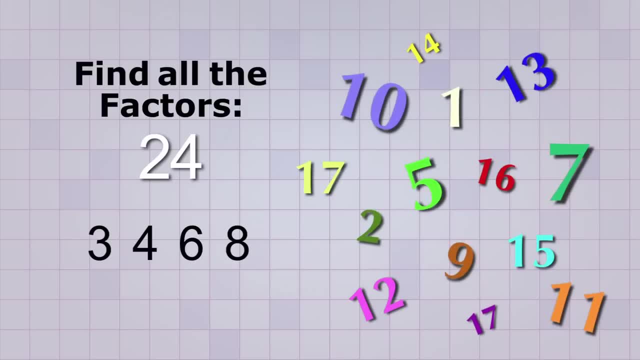 We already know 4 of them, but there's a lot more numbers we can test. Fortunately, we only need to test numbers that are less than HALF of the number we're testing And since half of 24 is 12, we just need to test the numbers 1 through 12.. 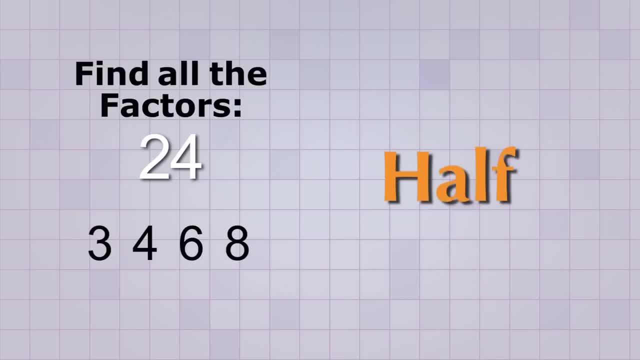 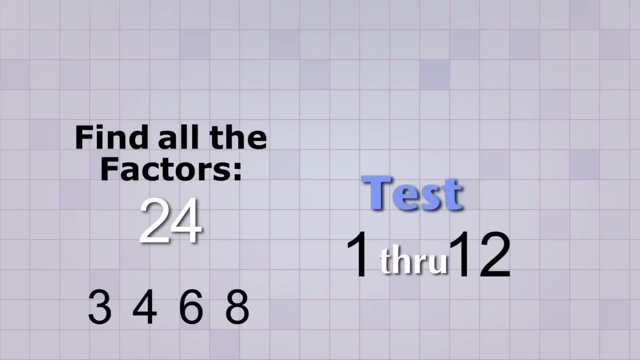 Fortunately, we only need to test numbers that are less than half of the number we're testing, And since half of 24 is 12, we just need to test the numbers 1 through 12.. To keep things organized, let's list the numbers we're going to test. 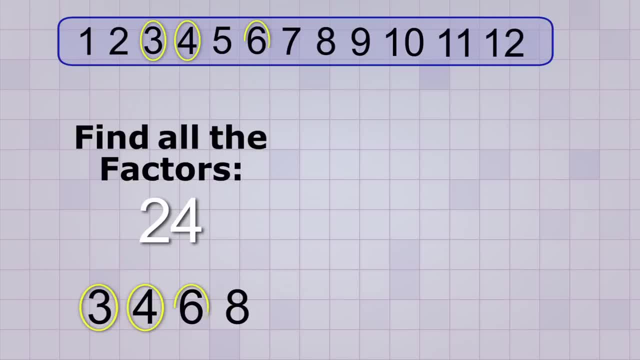 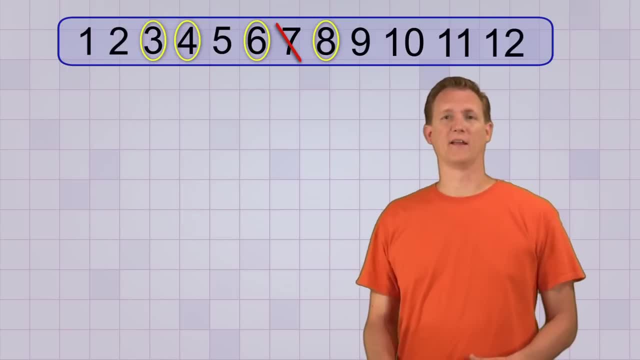 and we'll circle the factors that we already know: 3,, 4,, 6, and 8.. We can also cross out the 7, since we already tested it and found out it wasn't a factor. Okay, now for the numbers we haven't tested yet. Let's start with 1.. Well, of course, 1 is a factor. 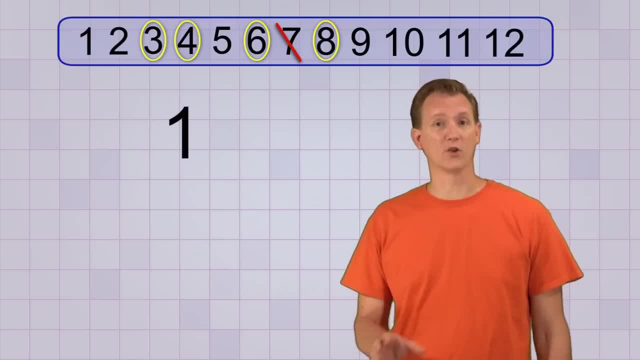 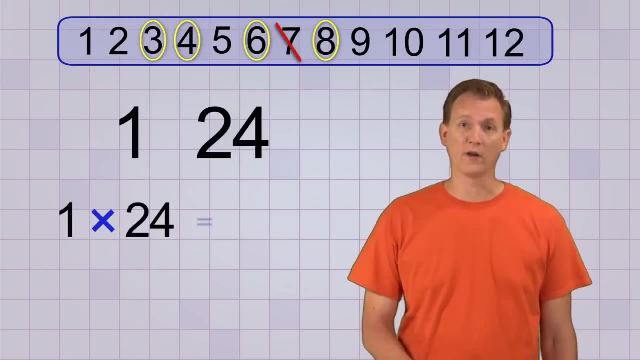 because 1 will divide evenly into any whole number. so 1 is always a factor. And since 1 is a factor, then that means that 24 is also a factor, because 1 times 24 equals 24.. It might seem weird that a number is always a factor of itself, but it's true. Knowing that helps you. 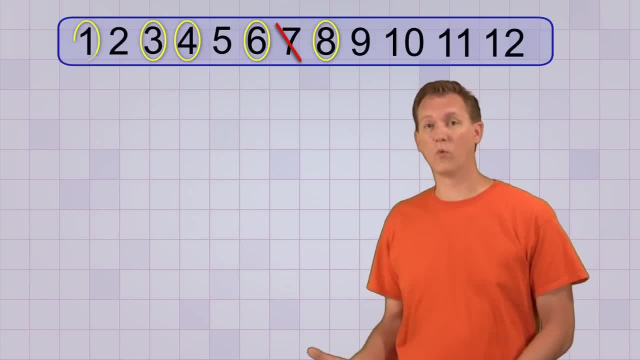 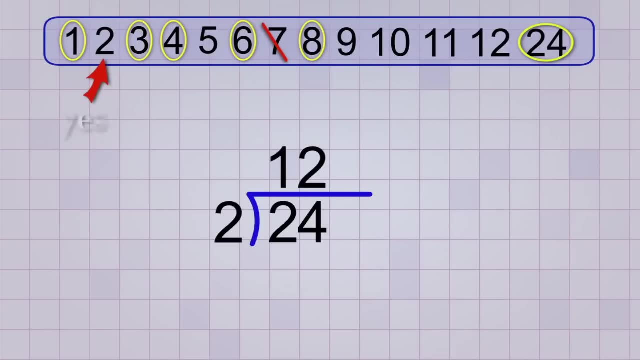 get started listing the factors, because you can ALWAYS include 1 and the number itself. Now let's move on and test 2.. If we divide 24 by 2, we get 12, so, yes, 2 is a factor, because it divided evenly. 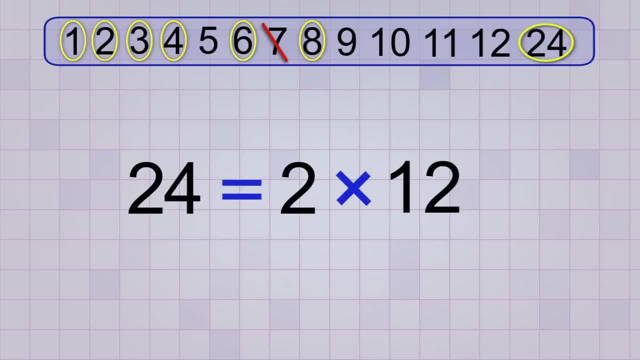 You can factor 24 into 2 times 12. That means that we can ALSO circle 12 as a factor of 24.. So any time you do a divisibility test and the number you're checking passes the test, then the answer you get from dividing- 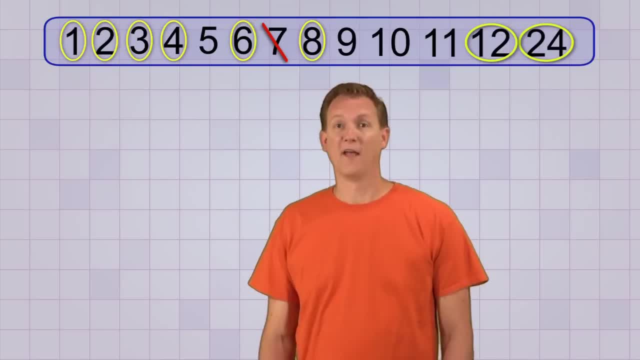 will also pass the test. However, will also be a factor That will speed things up, because we know we don't have to test 12.. Okay, let's move on to the next number. we haven't checked 5.. 24 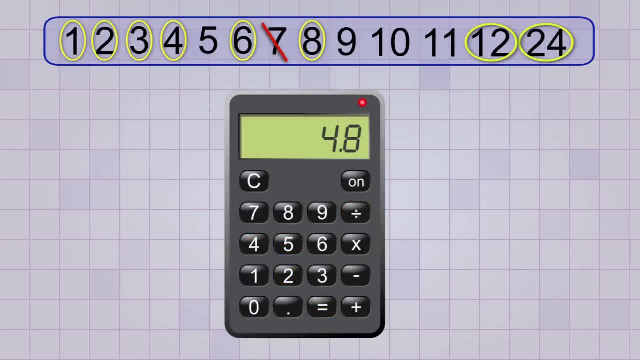 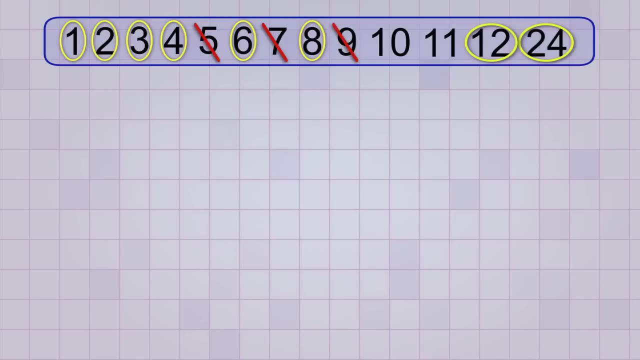 divided by 5 equals 4.8.. Well, that didn't divide evenly, because our answer is a decimal number. That means that 5 is not a factor of 24.. Next we'll try 9.. 24 divided by 9 equals 2.6666.. That's definitely not a factor. Okay, how about? 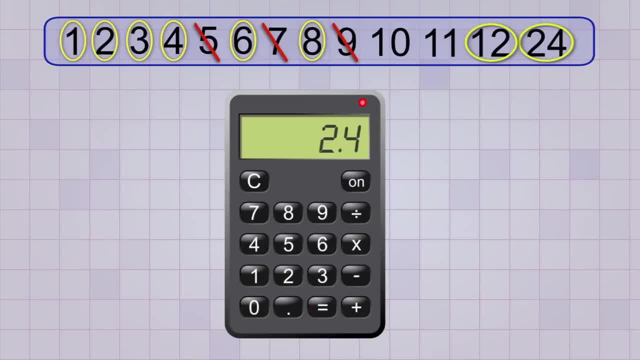 10. 24 divided by 10 equals 2.4.. Nope, that's a decimal number, so 10 is not a factor. It looks like the last one we have to try is 11.. 24 divided by 11. 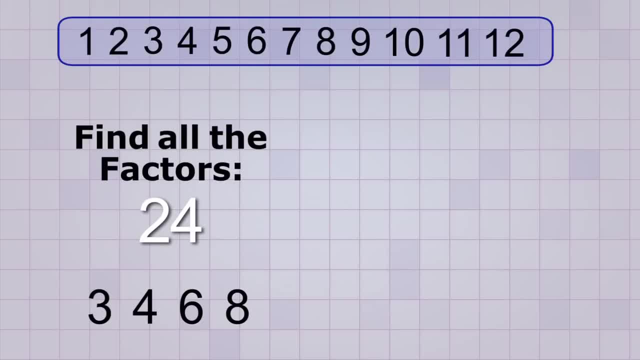 To keep things organized, let's list the numbers we're going to test and we'll circle the factors that we already know: 3,, 4,, 6, and 8.. We can also cross out the 7,, since we already tested it. 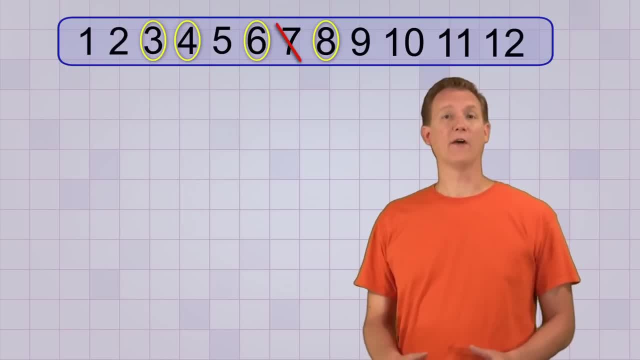 Okay, now for the numbers we haven't tested yet. Let's start with 1.. Well, of course, 1 is a factor, because 1 will divide evenly into ANY whole number. so 1 is ALWAYS a factor. And since 1 is a factor, then that means that 24 is also a factor, because 1 times 24 equals. 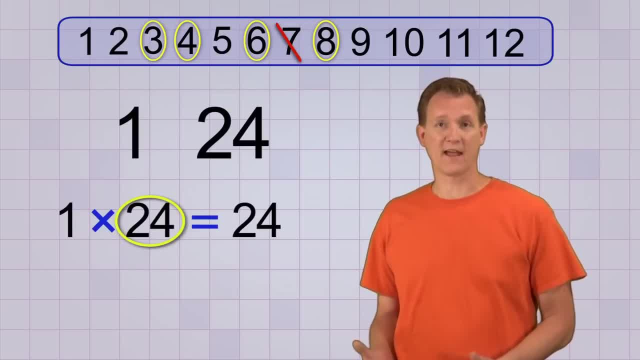 24.. It might seem weird that a number is always a factor of itself, but it's true. Knowing that helps you get started listing the factors, Because you can ALWAYS include 1,, 24, and 8.. So let's start with the numbers. we haven't tested yet. Let's start with the numbers. we haven't tested yet. Let's start with 1.. Well, of course, 1 is a factor, because 1 will divide evenly into ANY whole number. so 1 is ALWAYS a factor, because 1 is ALWAYS a factor. And since 1 is a factor, then that means that 24 is also a factor, so 1 is ALWAYS a factor. 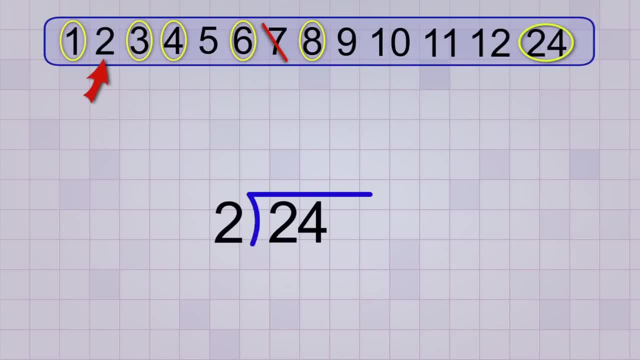 Now let's move on and test 2.. If we divide 24 by 2, we get 12.. So, yes, 2 is a factor, because it divided evenly. You can factor 24 into 2 times 12. That means that we can. 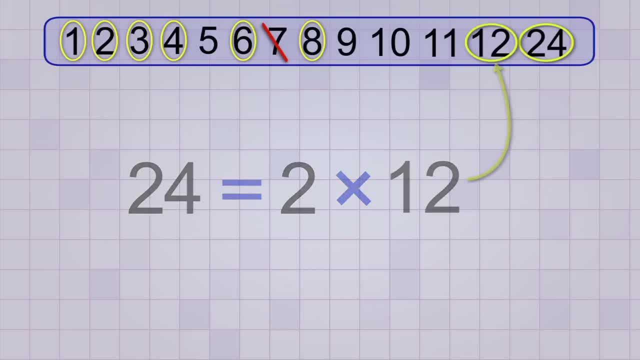 ALSO circle 12 as a factor of 24.. So anytime you do a divisibility test and the number you're checking passes the test, then the answer you get from dividing will also pass the test. It will ALSO be a factor That will speed things up, because we know 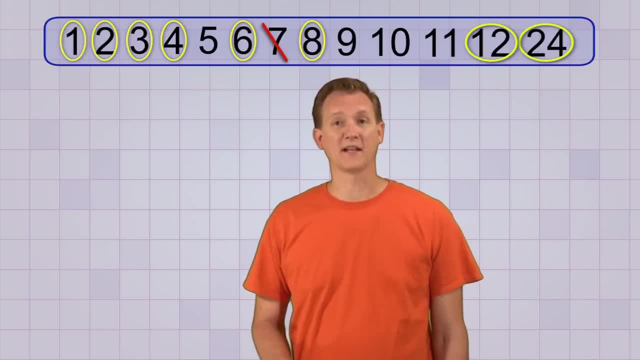 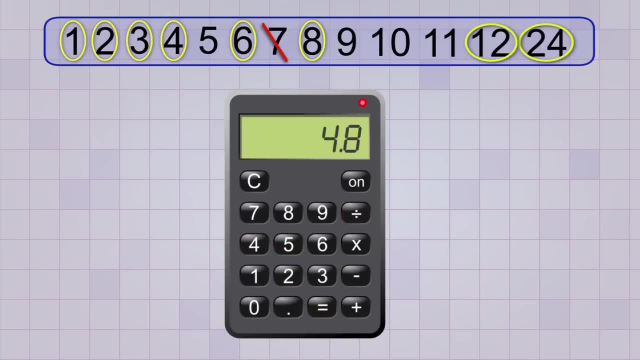 we don't have to test 12.. Okay, let's move on to the next number. we haven't checked 5.. 24 divided by 5 equals 4.8.. Well, that didn't divide evenly, because our answer is a decimal number. That means 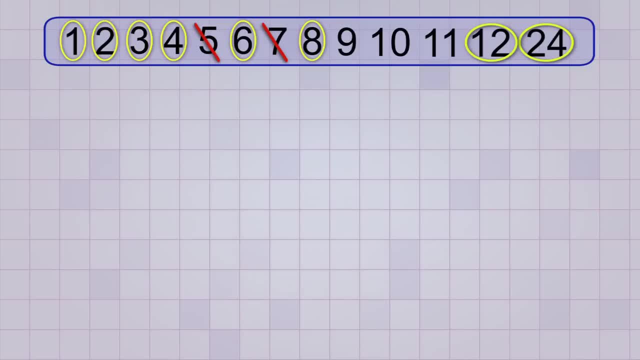 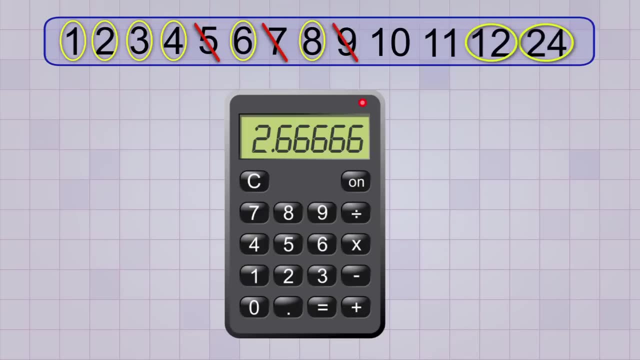 that 5 is NOT a factor of 24.. Next we'll try 9.. 24 divided by 9 equals 2.6666.. That's definitely not a factor. Okay, how about 10?? 24 divided by 10 equals 2.4.. Nope, that's a decimal number. 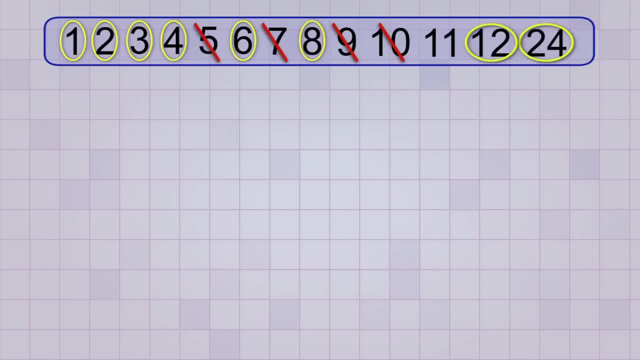 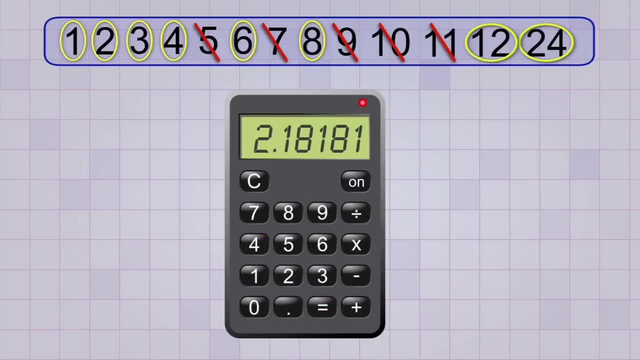 So 10 is NOT a factor. It looks like the last one we have to try is 11.. 24 divided by 11 equals 2.181818.. That's not a factor either. Alright, since we've tested all the numbers that are less than half of 24, we've found: